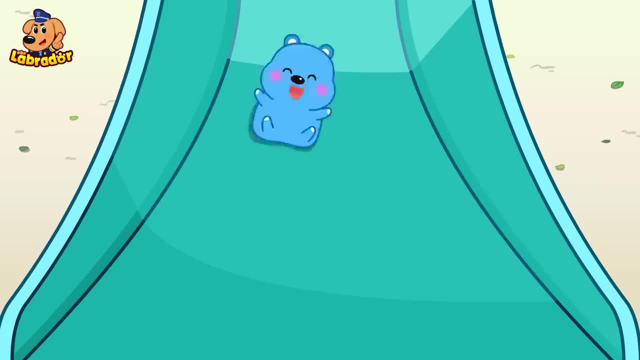 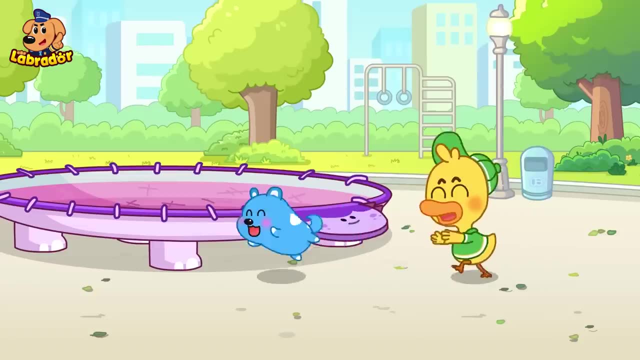 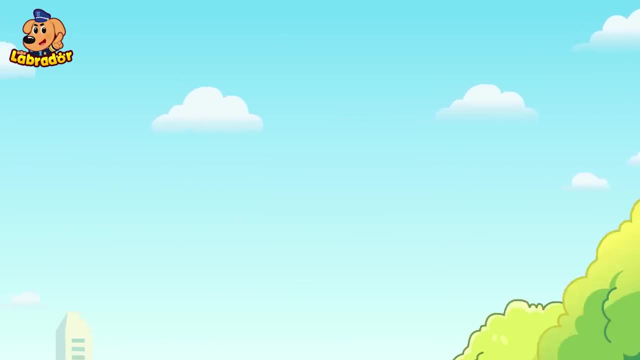 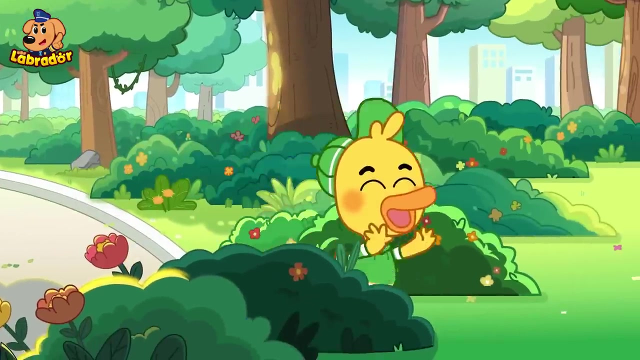 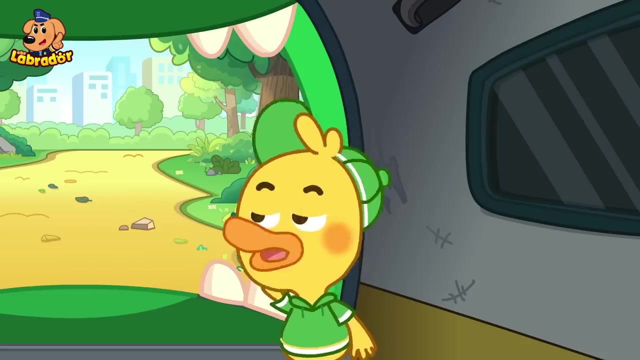 Lulu, Lulu, Lulu, Lulu. Wow, Play with me. Time to move. Lulu, Lulu, Lulu, Wait, Lulu Lulu. Little voice and little shape. Let me out. Drinked another cake. 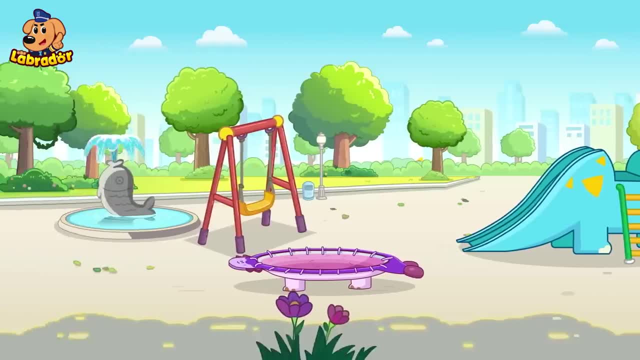 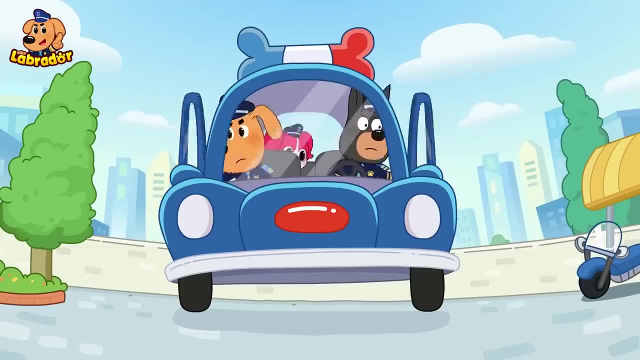 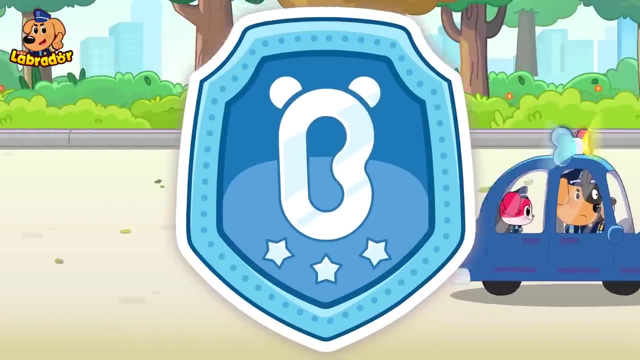 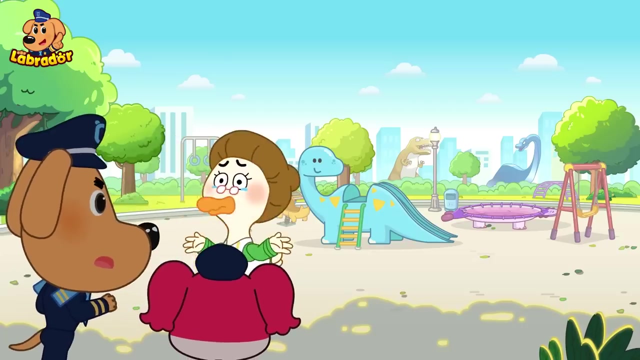 Sweety Grandpa's back. Aww, Little duck, Little duck, Ohhh, My grandson is missing. Oh, Oh, Oh, Sheriff Labrador, please help me find my grandson. He was just playing over there. Little slices, Little sheep. 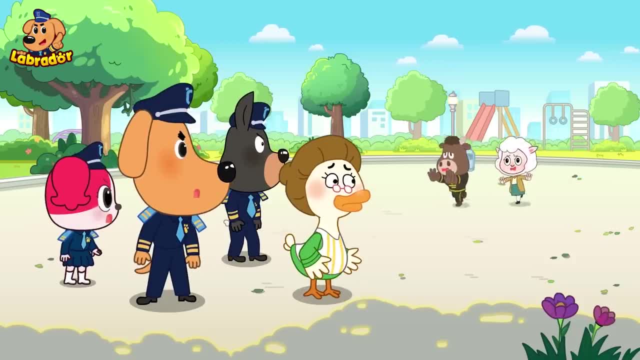 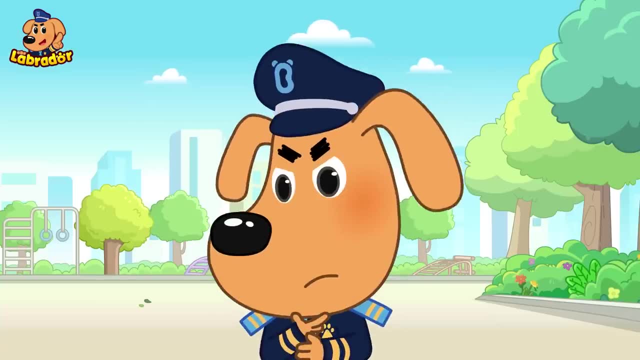 Shut it. insulation and some more begins that: う, Don't talk too loud here, Get off me, Vamos, Ven. sogar My son is missing, And my daughter too. Please help us. This might be a series of kidnapping cases. 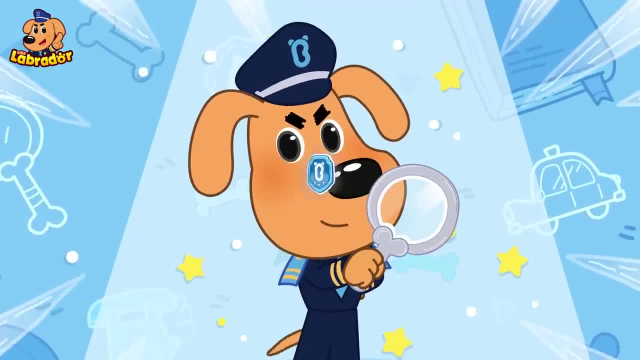 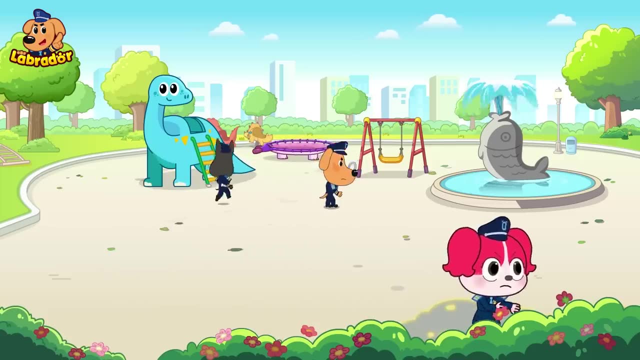 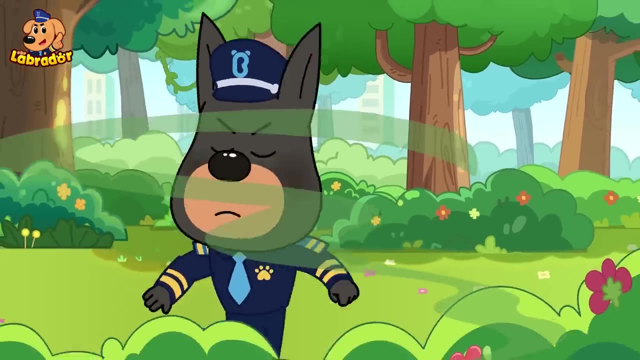 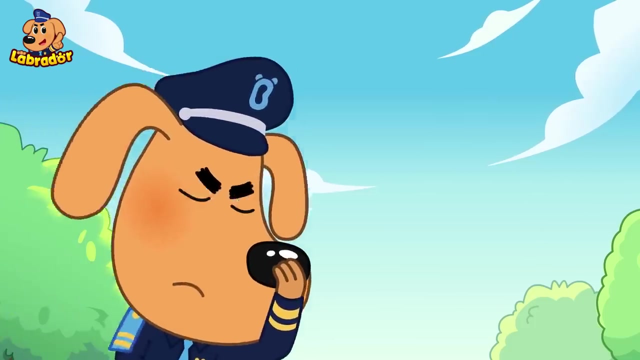 Don't worry, there's no case that I can't solve. Pacquiao Gobi. let's split up and investigate. Hey, What's that smell? It's poop. This is Pet Lulu's poop, Who didn't clean up their pet's poop. 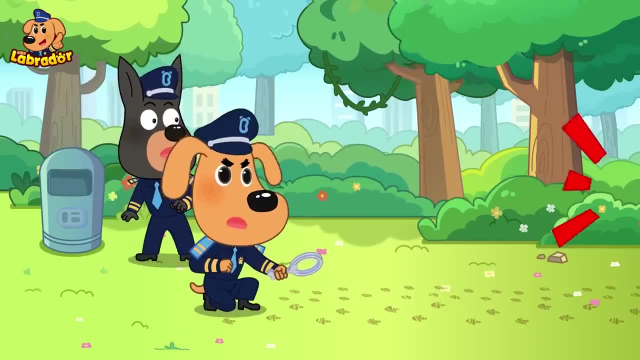 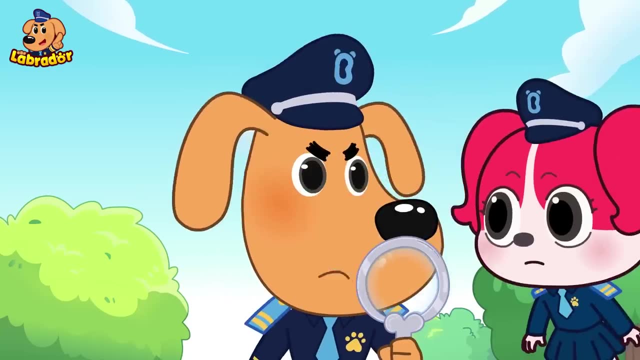 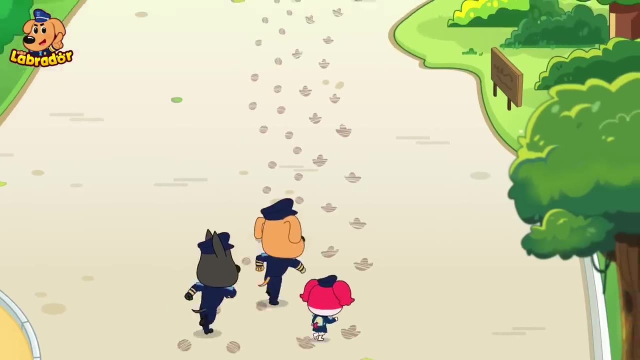 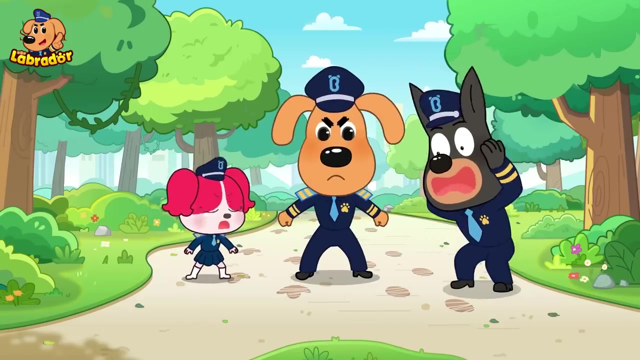 Little Duck and a Lulu's footprints. Sheriff Labrador, you should see this. According to the footprints, the kids were following the Lulu. I think someone used their pet to take the children. Follow the footprints. The footprints stop here. What do we do? 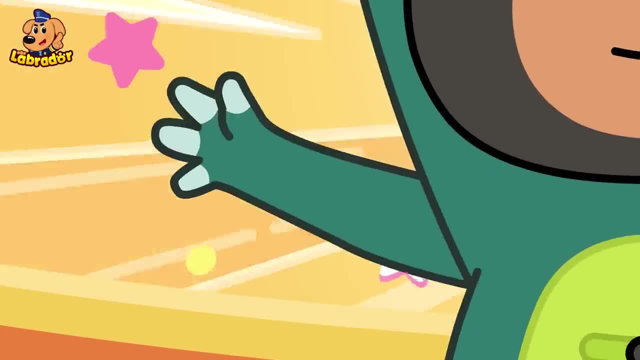 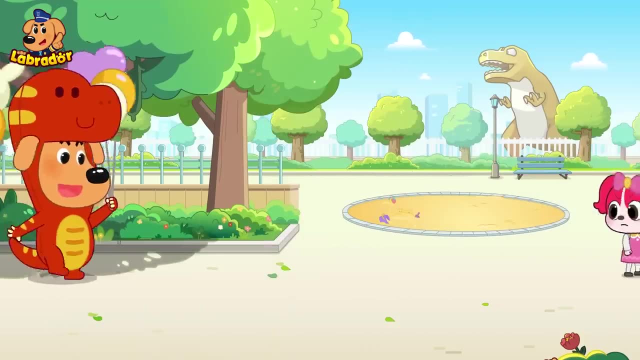 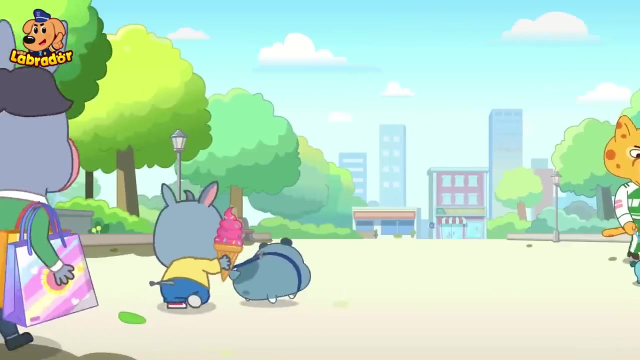 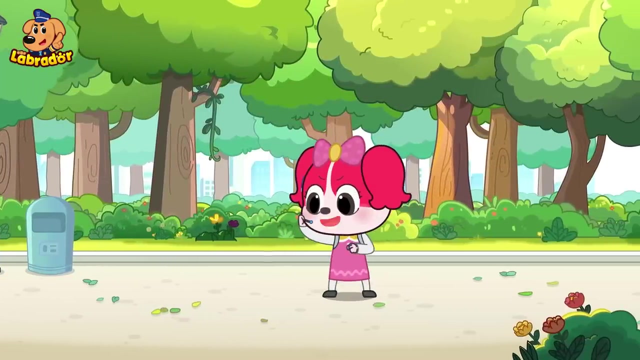 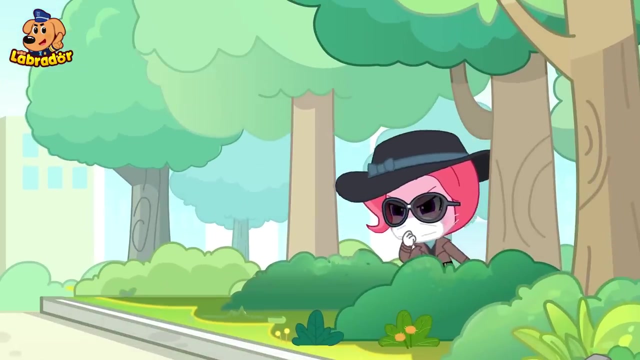 Don't worry, I have a plan. Three kids went missing in this park. The suspect might be nearby. No target found. Make some noise to attract the suspect, No problem. This is so fun. Another kid to trick Lulu go. 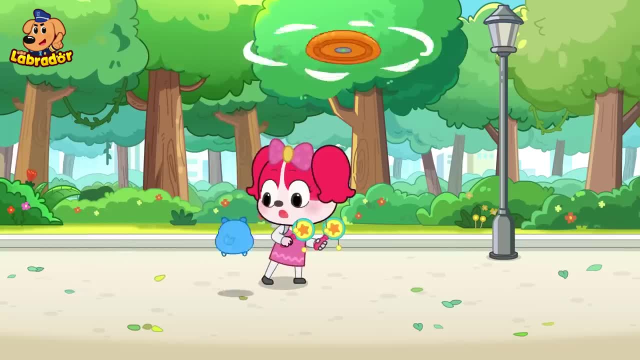 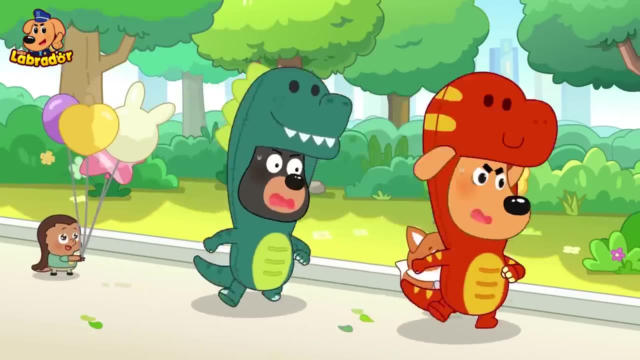 Lulu, Lulu, Lulu, Lulu. Sir, it's trying to get my attention. This might be the suspect's Lulu. Follow it, It'll lead us to the missing kids. It ran away. Don't lose it. 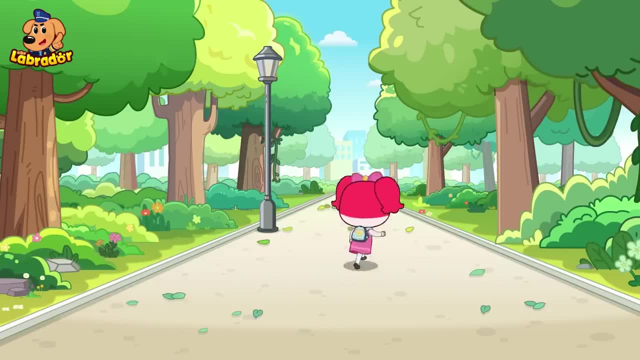 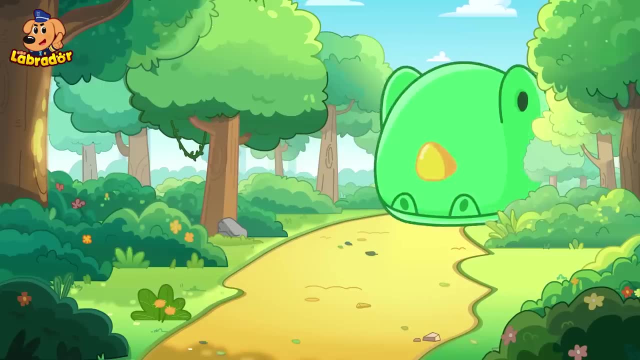 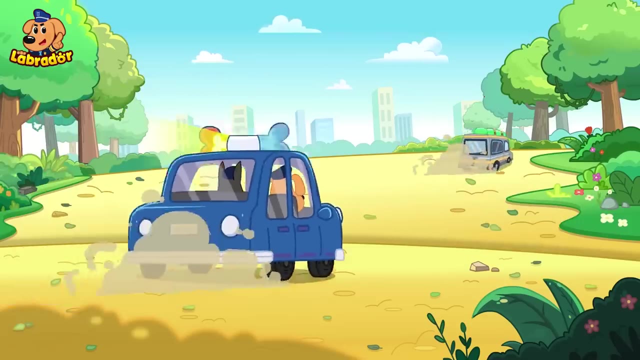 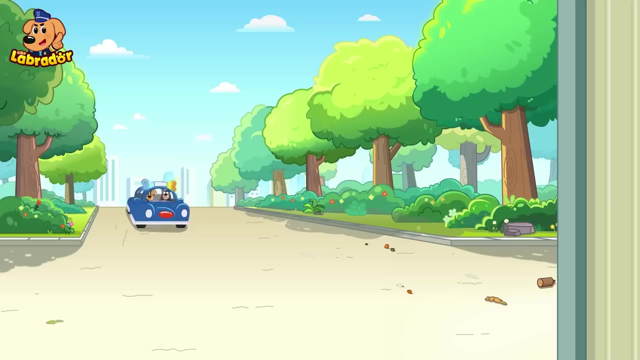 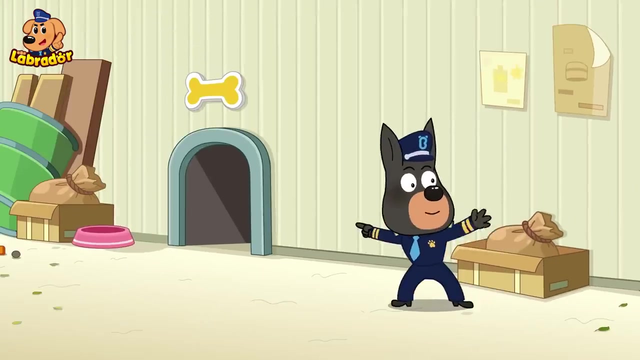 Okay, Lulu, Lulu, Follow that car. The door is closed. The door is closed. Oh, Look, There's another door. Hmm, Oh, Oh, Tobi, get back. Oh, That was a mistake, Oh. 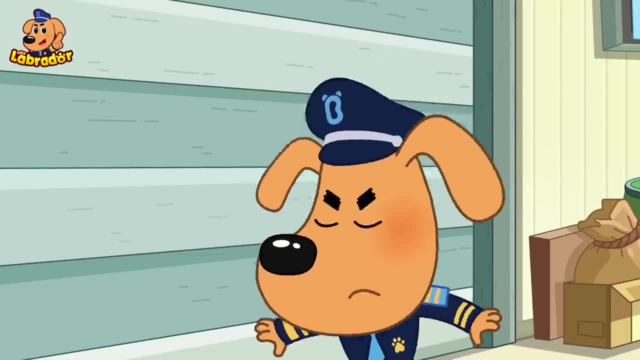 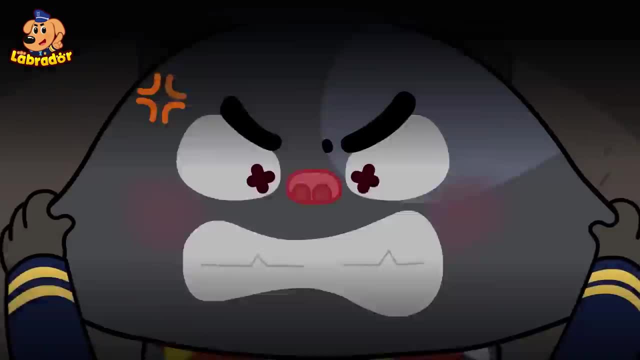 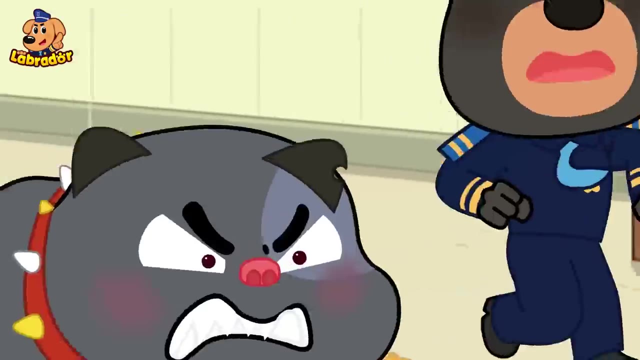 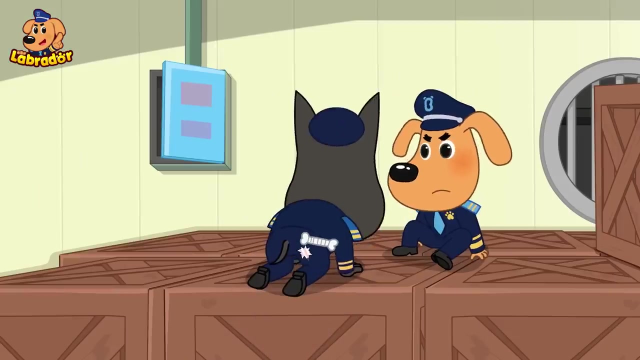 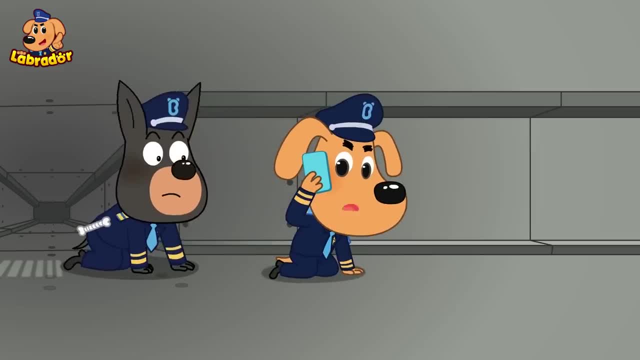 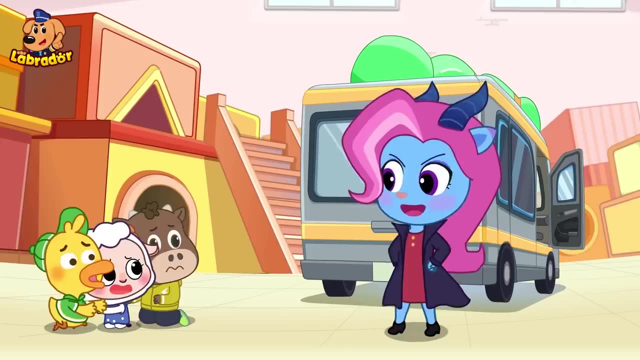 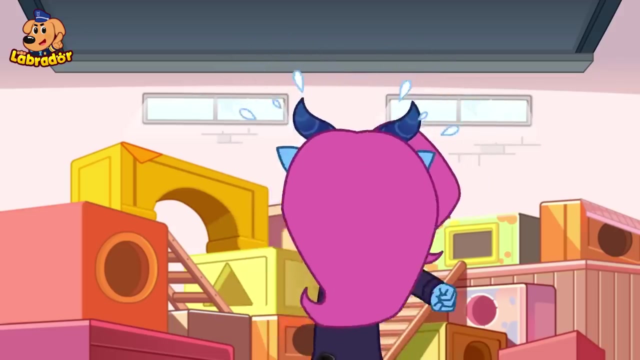 Sir, I found the missing kids. Be careful, we'll be right there. Whoa, Oh, what a lucky day. It's you again, Antel, Oh the police, Oh no, You won't get away, Oh Sheriff Labrador. 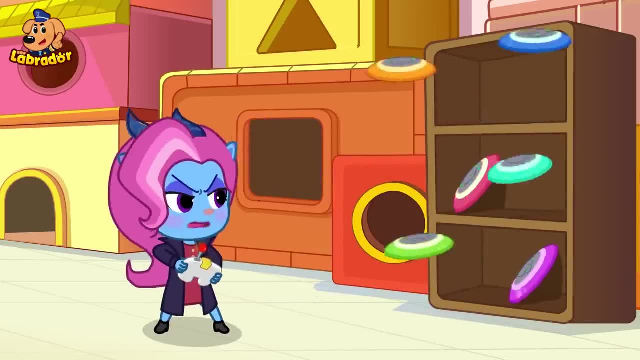 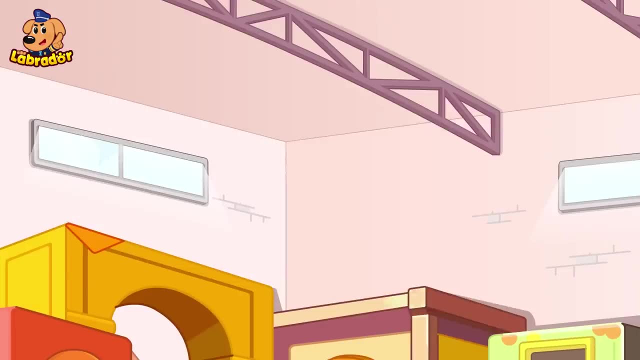 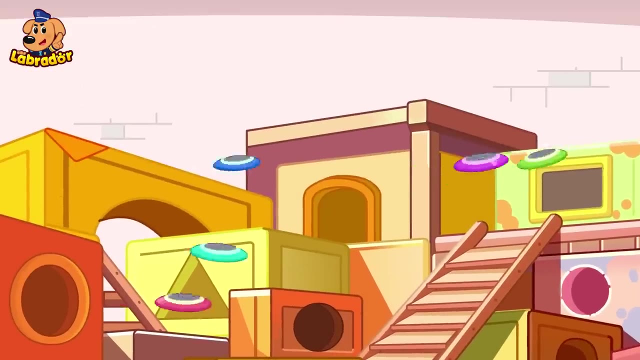 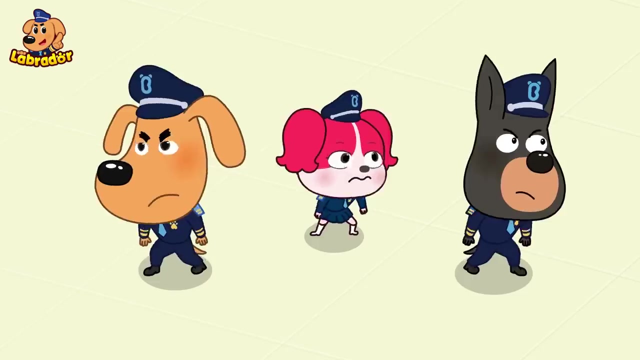 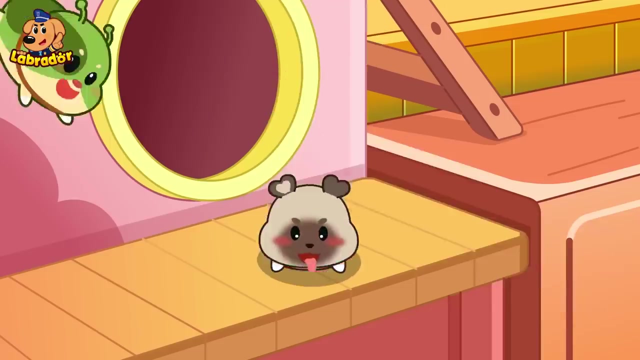 It's okay now. You'll never catch Dr Antel. They won't stop us. I'm smarter than you think. Lo-Lo, Lo-Lo, Lo-Lo, Lo-Lo. Go My loulous Lo-Lo, Lo-Lo.